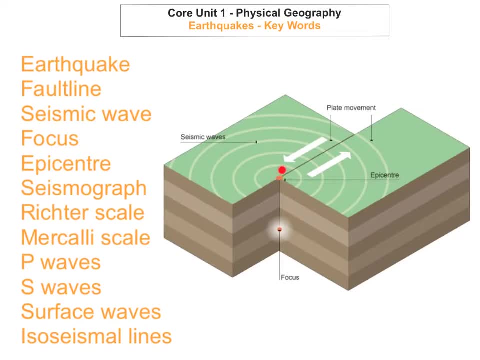 So one thing to know is that the strength of these like seismic waves is measured by an instrument called the seismograph, And the seismograph basically just detects and records and measures earthquakes, And they usually do this on then on the Richter scale. 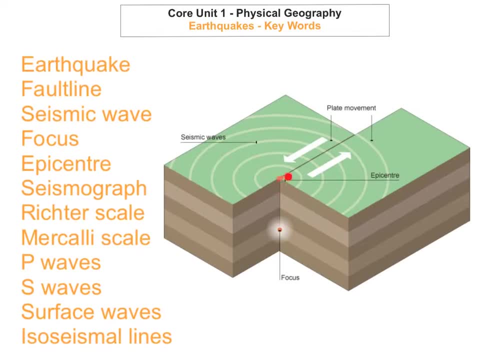 One thing to note: the person who actually studies earthquakes, or the study of earthquakes, is called seismology. So seismology is a study of earthquakes. The Richter scale, this is a way to actually measure earthquakes. So with the Richter scale, it determines the magnitude of the seismic waves. 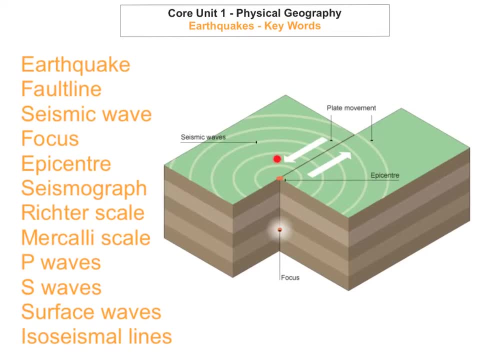 And it's done in each unit. increases on the scale means that it's the seismic waves are ten times as large. Okay, so, for example, if it was like seven on the Richter scale And the seismic waves were ten times larger than the earthquake, that suffered six on the Richter scale. 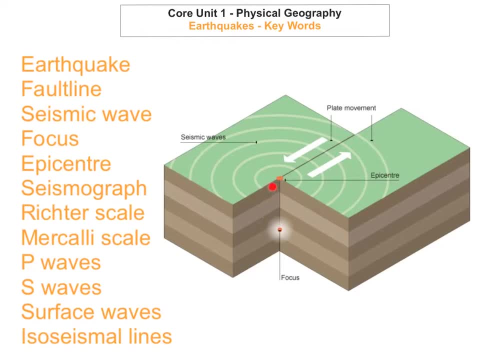 So it's really important to know. So if it's seven on the Richter scale and another earthquake is eight on the Richter scale, Well that means that's ten times stronger. The next one is the Macaulay scale, and the Macaulay scale is the same as the Richter scale. 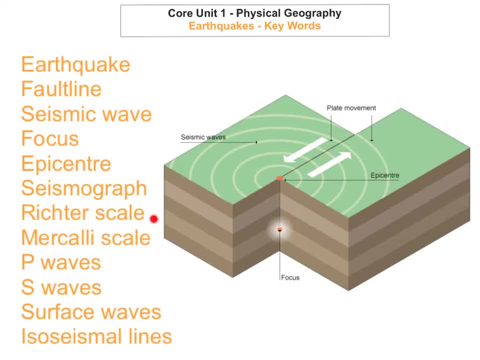 It measures like the intensity of earthquakes, but it's done by description. So basically, people in the area have to, they have to basically rate the amount of destruction, But like through observations. So it's another way to measure the intensity, but it's all done through observations. 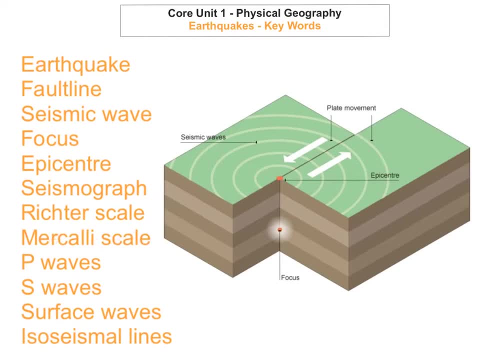 And how much damage is observed and is actually done. The next one is P waves. So P waves are primary waves, So these P waves are the first waves to arrive And they travel through both solid and molten materials of the Earth's interior. 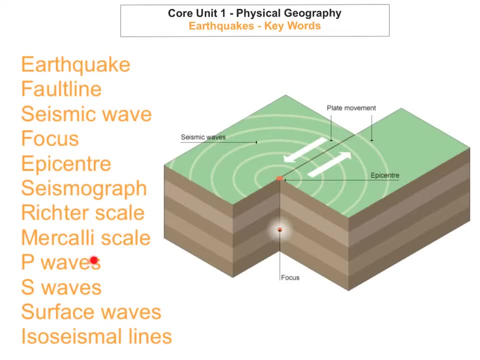 And cause rocks to vibrate back and forth in the direction of the wave motions. Okay, The wave motion S waves are sometimes known as secondary waves, So they move at about half the speed of the P waves And they move only through solid rock.